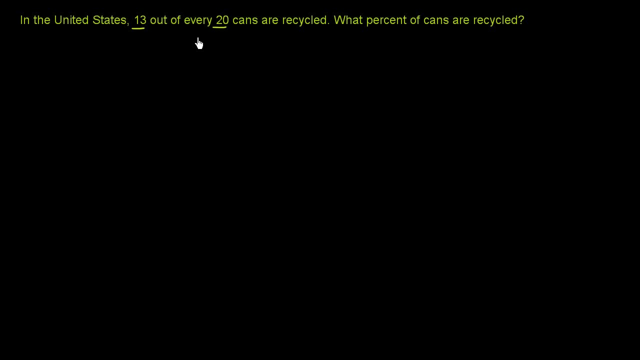 In the United States, 13 out of every 20 cans are recycled. What percent of cans are recycled? So 13 out of every 20 are recycled, So 13 20ths or 13 over 20, could also be viewed as 13 divided by 20, or 13 divided by 20.. 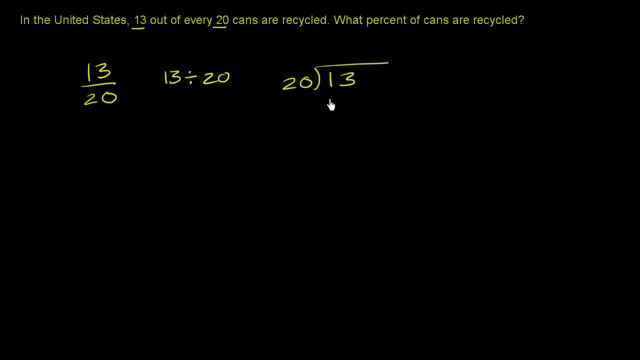 And if we do this we'll get a decimal, And it's fairly straightforward to convert that decimal into a percentage, So 13 divided by 20.. We have the smaller number in this case being divided by the larger number, So we're going to get a value less than 1.. 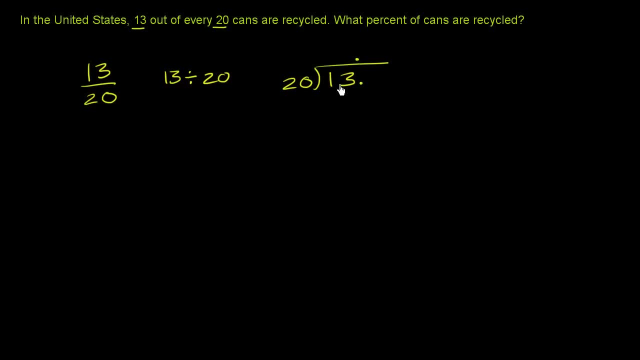 Since we're going to get a value less than 1, let's put a decimal right over here And let's add a couple of 0s- as many 0s as we would need- And we could say: hey look, 20 goes into 13 0 times. 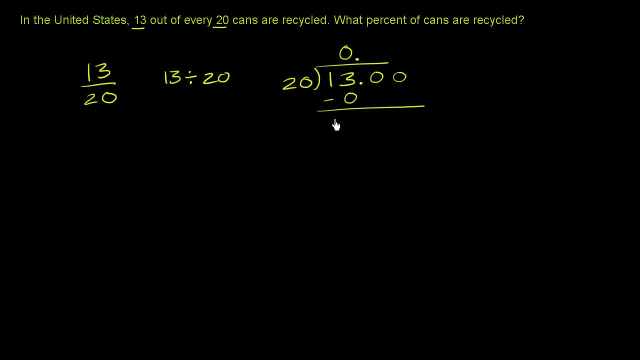 0 times 20 is 0. And then 13 minus 0 is 13.. Now you bring down a 0.. 20 goes into 130.. Let's see: 5 times 20 is 100.. So 6 times 20 is 120.. 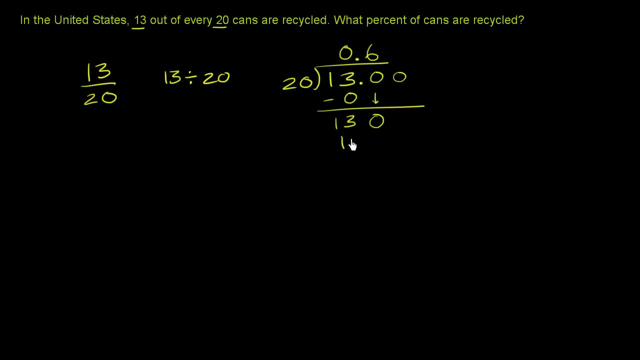 So it's going to go 6 times. 6 times 20 is 120.. You subtract, You get a 10.. Let's bring down another 0.. 20 goes into 100. 5 times 5 times 20 is 100.. 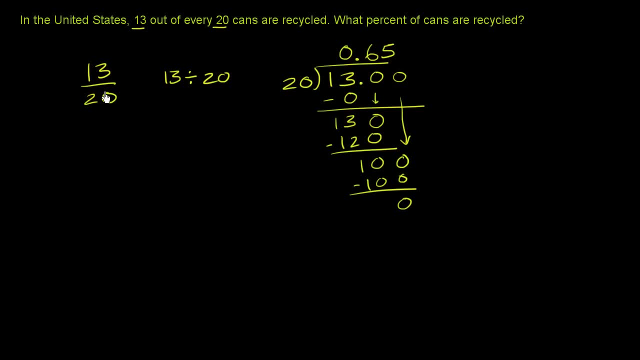 And we are done. So this written as a decimal, It's 0.65.. So as a decimal, it's 0.65.. And if you want to write it as a percentage, you essentially multiply this by 100. Or another way you could say is you shift the decimal. 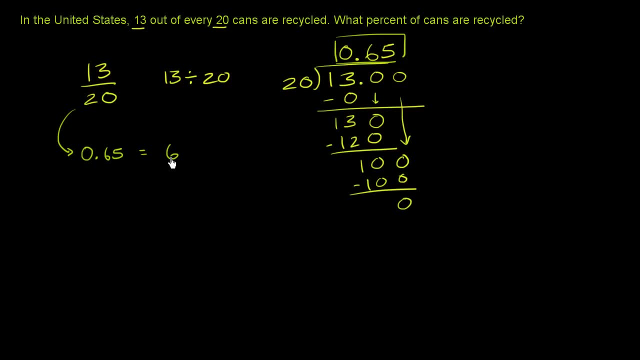 over two spots to the right. So this is going to be equal to 65%. Now there's another way you could have done. it Is you could have said: look, percent literally means per 100. So 13 out of 20.. 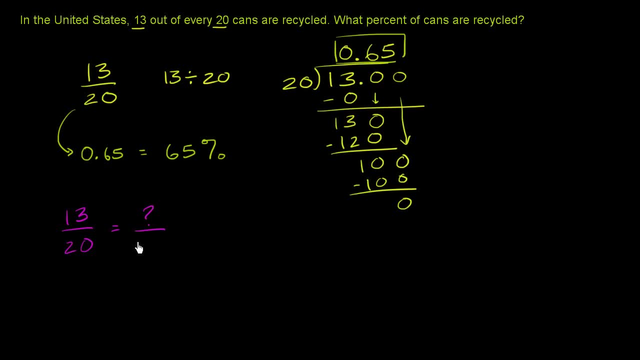 So 13 out of 20 is going to be equal to what? over 100?? Well, to go from 20 to 100, you get the denominator. To go from 20 to 100, you would multiply by 5.. So let's multiply the numerator by 5 as well. 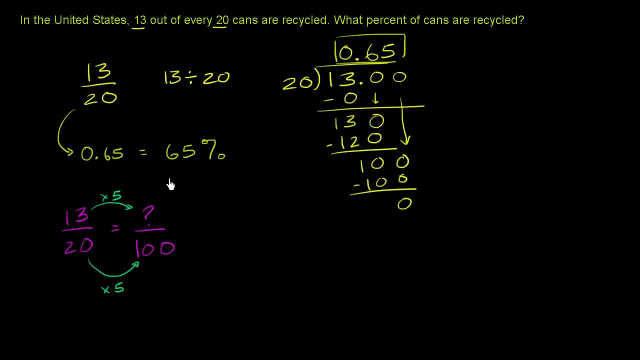 And 13 times 5.. Let's see that's 15 plus 50, which is 65. So this would have been a little bit of a faster way to do it, Especially if you recognize it's pretty easy to go from 20 to 100.. 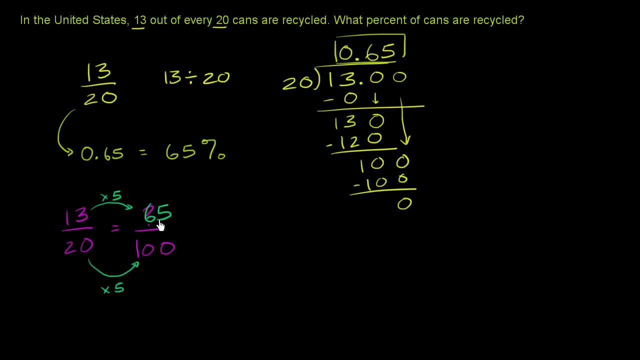 You multiply by 5.. So we would do the same thing with the 13. And so you'd get 65 over 100, which is the same thing as 65 per. let me write this percent symbol: 65%, And just a reminder: percent literally means per 100. 65 per 100, 65%. 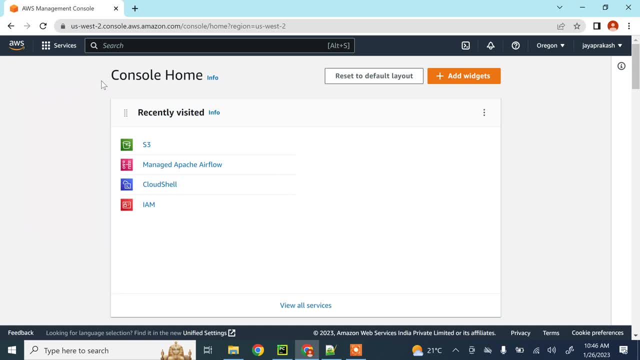 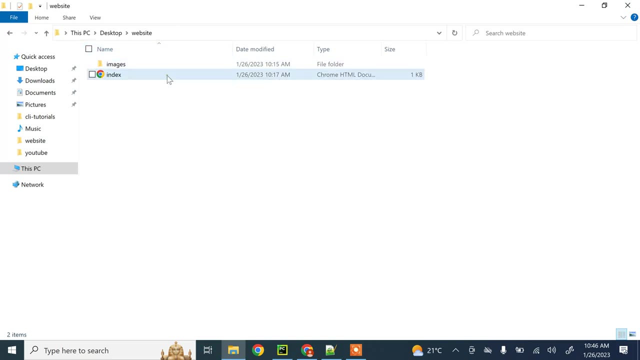 Hello everyone, In this video I'm going to show you how to host a static website on AWS S3.. So, for demonstration, I'm just going to build a very simple website and show you how to host it on AWS S3.. So let's get started. So this is my sample website. Like it's a very simple. 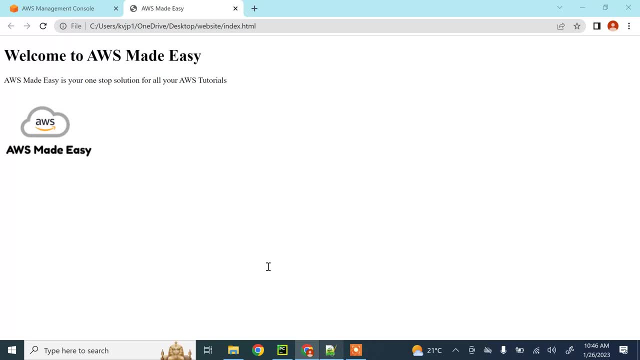 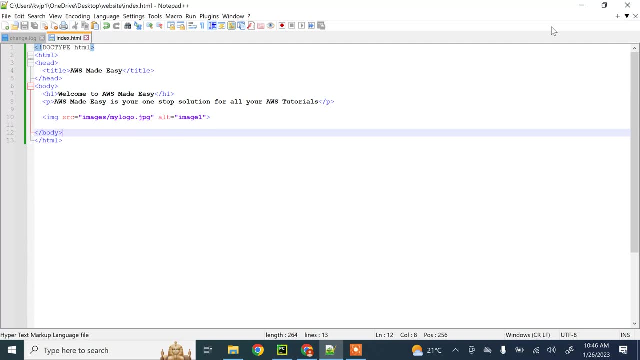 it has some text and I also have a logo here. So if you see my indexhtml, this is how it looks. I just have one- I mean some text- and one image. So, like I mean, you can host any static website. 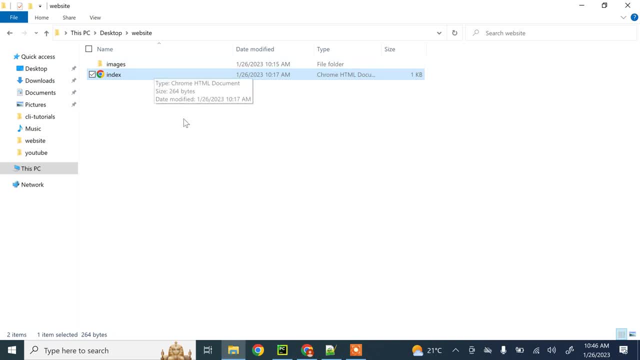 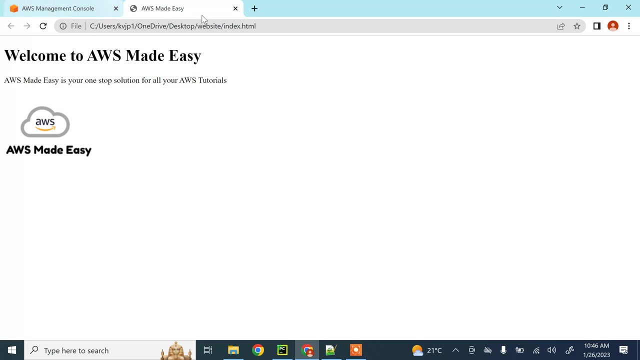 with text and multimedia videos, images as well. Okay So, but for demo purposes, I'm just going to host this simple website on S3 and show you how to do that. Okay So, once you have all the files needed for your website ready, you can navigate to AWS Management Console and click on S3. 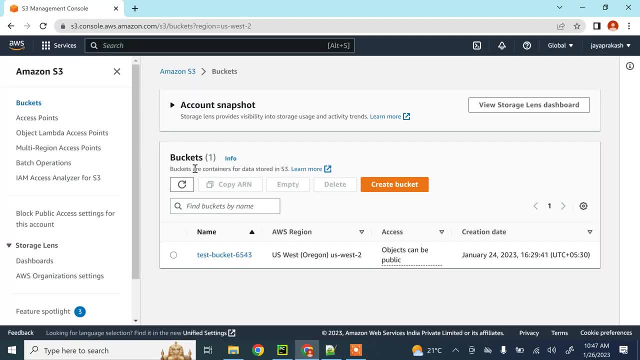 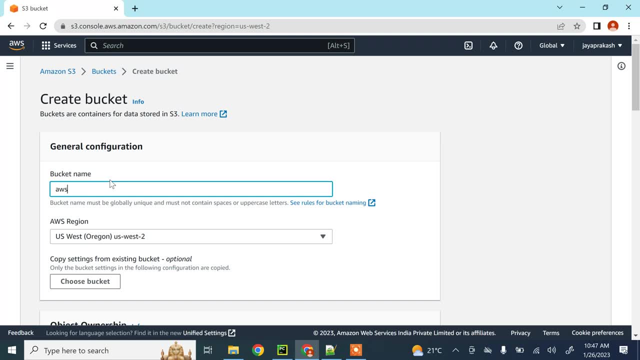 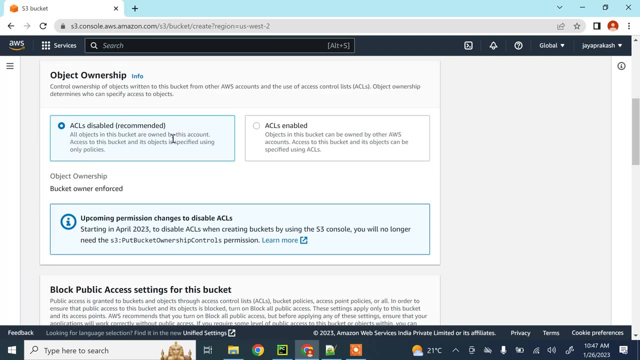 So we first need to create a bucket to host our website. So I'm going to select this bucket, So I'm just going to name it AWS Made Easy website And for now I'm just going to leave all the settings as default and create the bucket. Okay, We will need to change some settings later, So 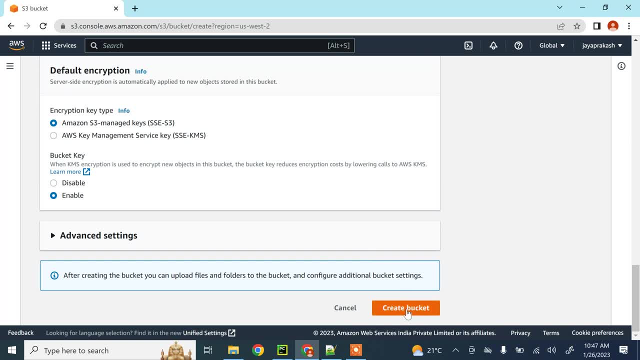 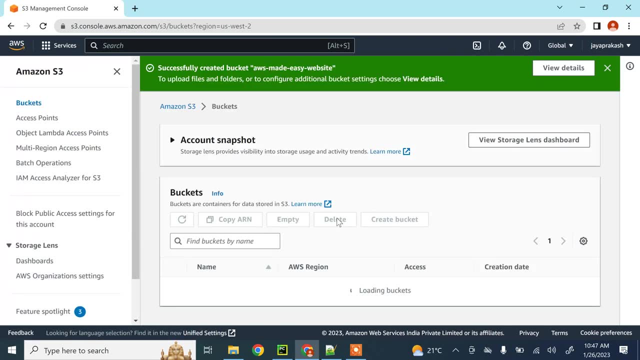 but we will see how to do that at a later point. Okay, So, for now, I'm going to create a bucket with all the default settings. Okay, So, once you have your website created, you need to upload all your files related to your